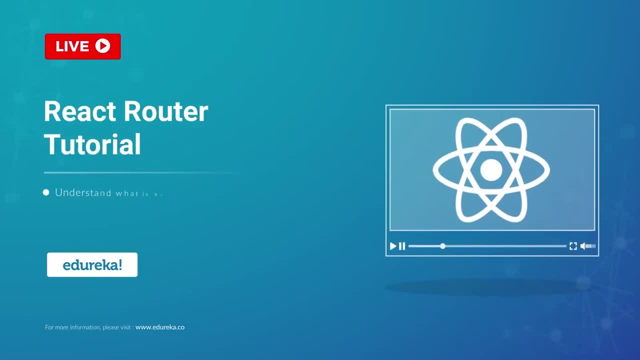 Components are the heart of react's powerful declarative programming model. react router is a collection of navigational components that compose declaratively with your application, whether you want to have bookmarkable URLs for your web applications or a composable way to navigate in react. native react router works. 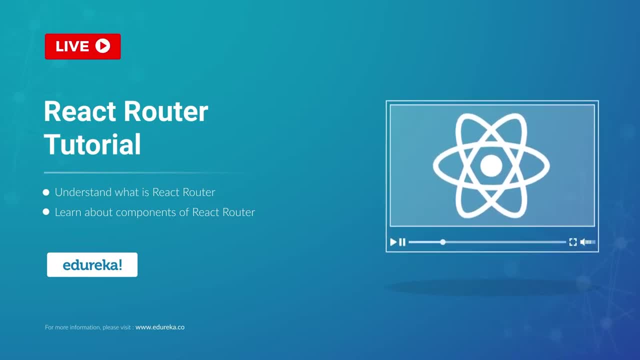 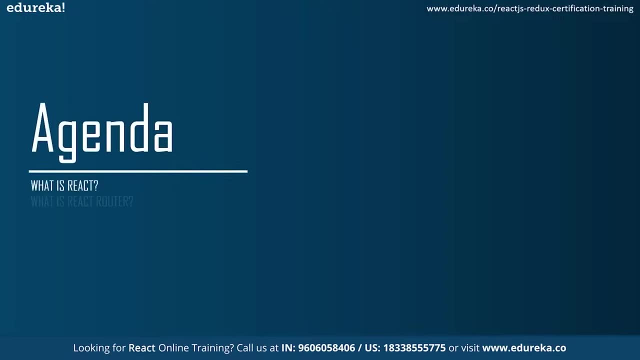 wherever react is rendering. Hello everyone, I'm Anika from Edureka. Welcome you all to the session on react router. before starting the video, Let me take you through the agenda of today's session. I will begin with discussing about what is react. moving on, I will discuss react router and then we'll see some of the advantages of using react router. Then I will show you how to install and set up the environment to use react router. afterwards We'll see the different components of react router and before wrapping up the session, I will discuss 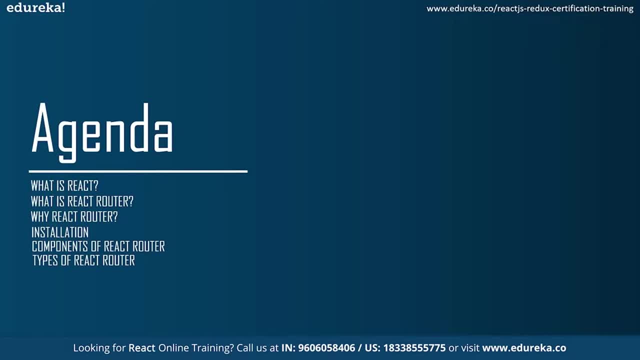 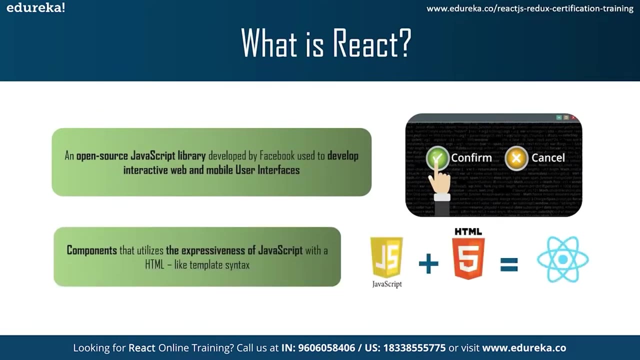 the types of react routers used, along with explanation. I will show you the demo also, which will ultimately lead to a small react application using react router, starting with what is react JS? So react is a JavaScript library, which means it is a collection of code on which many developers are working. for the last ticket. It allows us to build user interfaces for websites and also for other applications like mobile applications, desktop application and VR applications. Basically, 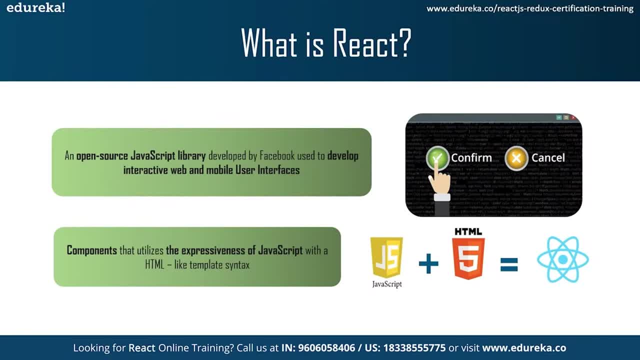 react is more concerned about building interfaces so that the users can interact with, getting data from the users and then display the information. so I can sum up: react as an open source JavaScript library developed by Facebook, used to develop interactive web and mobile user interfaces, and it is component based, where the components that utilizes the expressiveness of JavaScript with the HTML, like template syntax, are used. Now, before explaining react router, I would like to 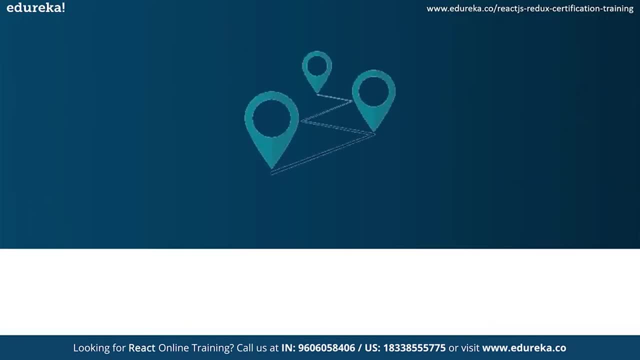 to give you a brief to routing. So routing is the ability to move different parts of an application when a user enters a URL or clicks an element like link button, icon, image, etc. within the application. routing is basically required in transitioning from one view to another in an application. 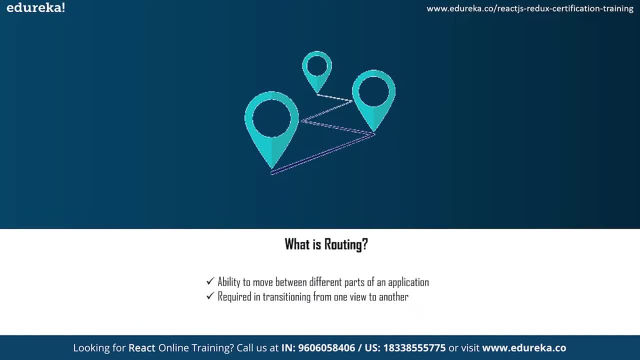 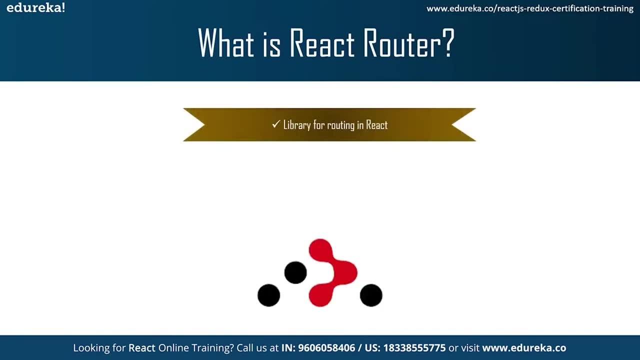 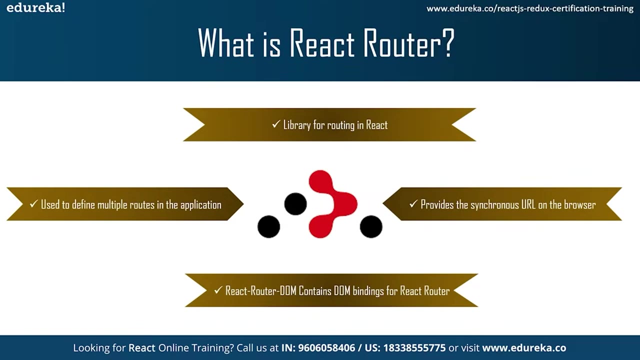 in simple words, I can say: routing is a process in which a user is directed to different pages based on their action or request. Now we are good to go to understand react-router. react-router is a standard library system built on top of the react and used to create routing in the react application. 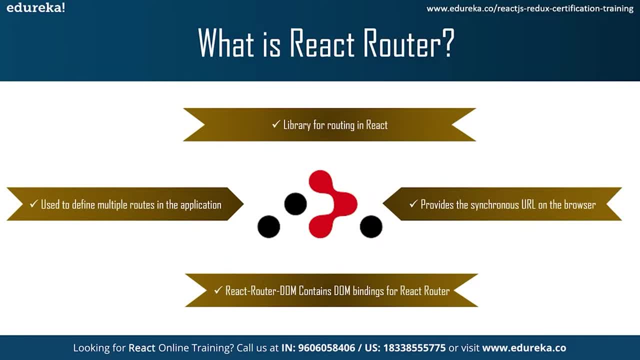 using react-router package. It provides the synchronous URL on the browser with data that will be displayed on the webpage. It maintains the standard structure and behavior of the application and mainly used for developing single-page web applications. It enables the navigation among views of various components. 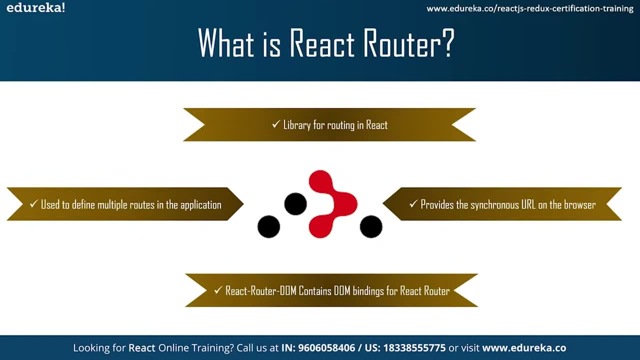 in a react-router. That application allows changing the browser URL and keeps the UI in sync with the URL. reactions router is mainly used for developing single-page web applications and it is used to Define multiple routes in the application when a user types of specific URL into the browser. 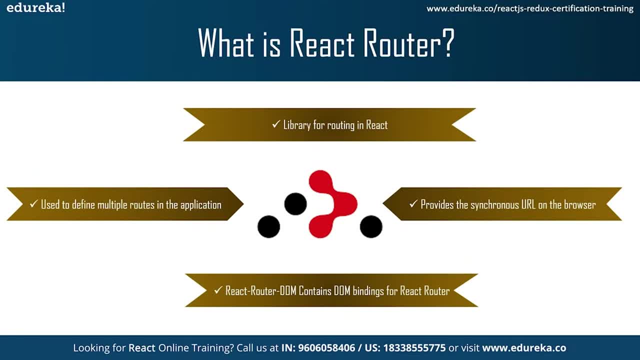 and if this URL path matches any route inside the router file, the user will be redirected to that particular room. react-router plays an important role to display multiple views in a single-page application, and without react-router It is not possible to display multiple views in react applications. 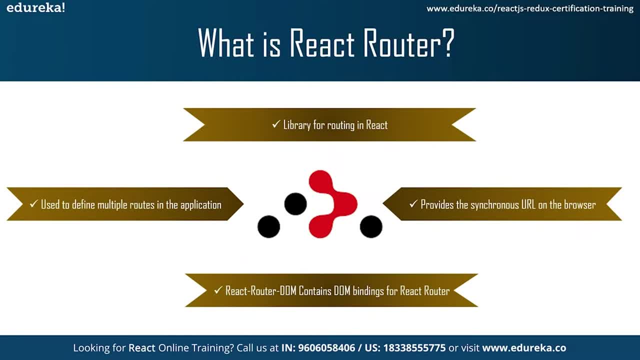 Most of the social media websites like Facebook, Instagram, Twitter, Airbnb, Etc. uses react-router for rendering multiple views, to make use of react-router, We have something called as react-router Dom. What is this react-router Dom, which is actually the react-router data object model? 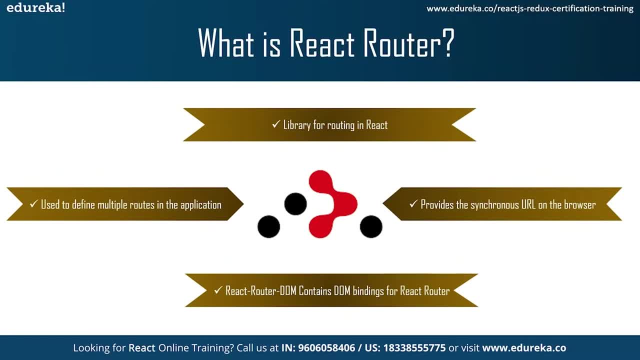 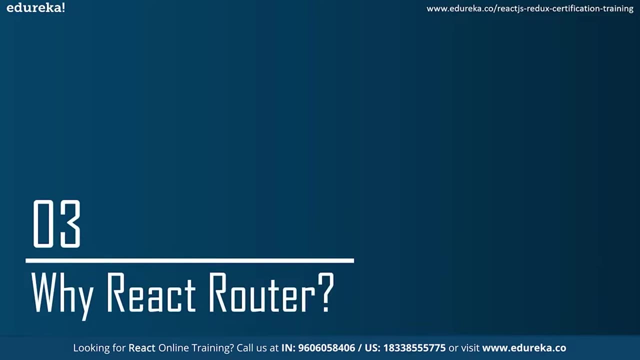 It contains the Dom bindings for react-routers, In other words, the router components for a websites. and if we talk about react-router native, it contains the react native bindings for react-router. the moving ahead. Let's see the advantages of react-router, because of which we are using react-router. 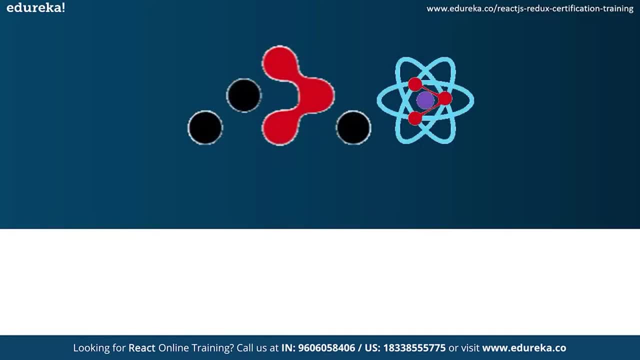 So in react-router it is not necessary to set the browser history manually and link is used to navigate the internal links in the application. It is similar to the anchor tag, which we know is very simple as we have learned in HTML. It uses switch feature for entering. 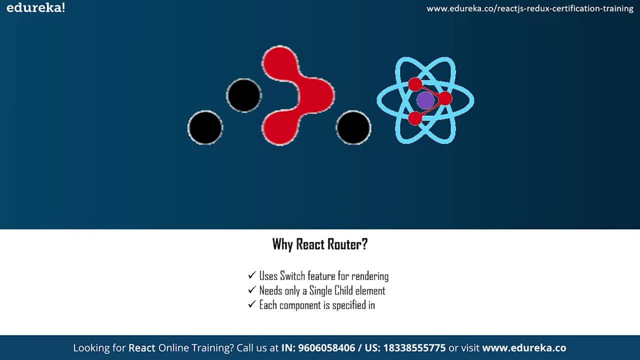 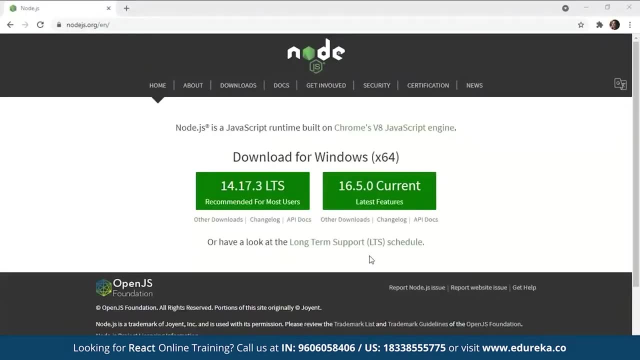 and the router needs only a single child element, so no complexity at all. and in react-router every component is specified in now talking about the installation part. So what we can do is we can just go to our nodes official website and we can just download the nodejs. 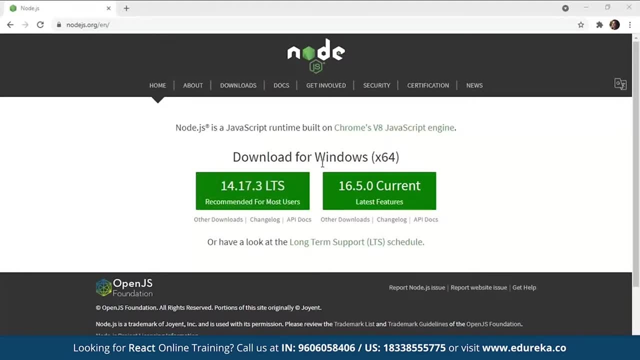 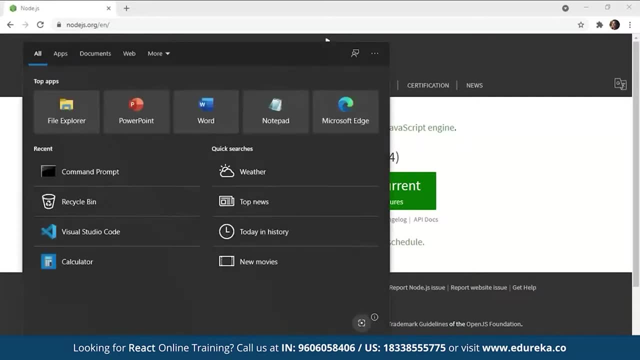 whatever the configurations of your windows are, We can just download it And once we have set up a nodejs on our PC, what we'll do is we will just install. create react app. Okay, that will be very helpful. while creating the application. 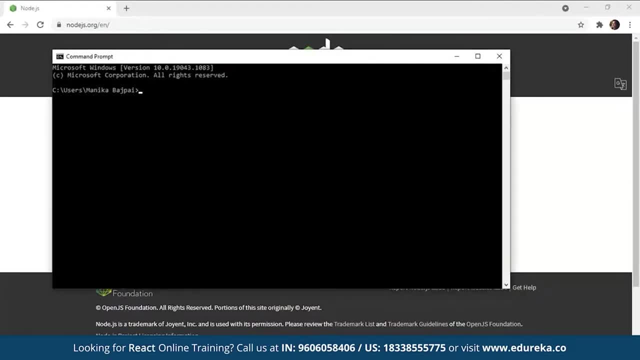 the demo which I am going to show you in the later part of the video. in that it will be very helpful. The command to install create react app is: npm. install hyphen G, then create hyphen react hyphen app. I'll just click on this. 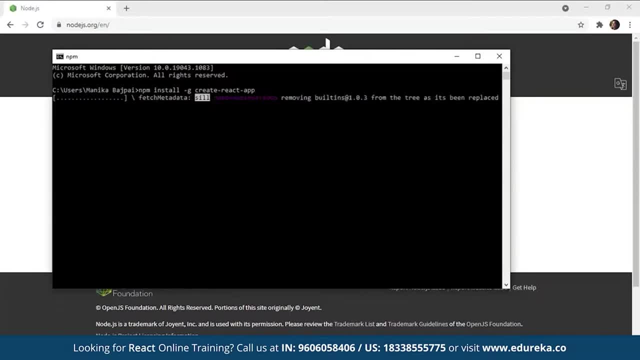 and this is how it is going to install: create react app. It will take quite some time, but I already have it installed So I do not need it. So I'll just stop this thing over here And after that, when we will start off with our demo part. 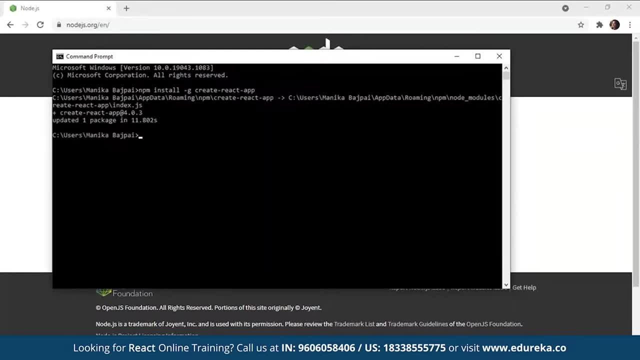 we will execute one more command that will be NPX- create react app- and will give the application name that we will see in later part of the video, when we'll start off with the demo part while creating the application itself. So this is what you have to do. 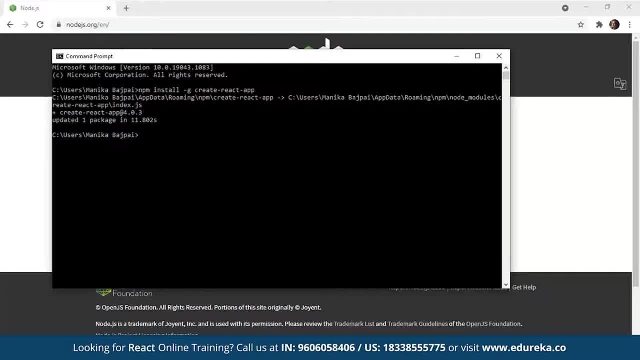 Then you will have to go to the directory where you have created the application, the folders. So with this we have successfully installed our create react application, which will help you to directly create and react application. We can just add the components to that. We can change the code. 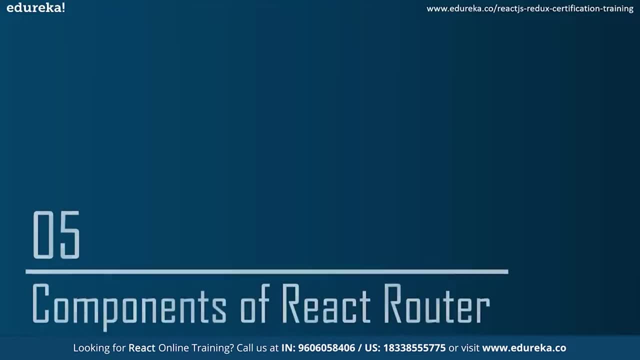 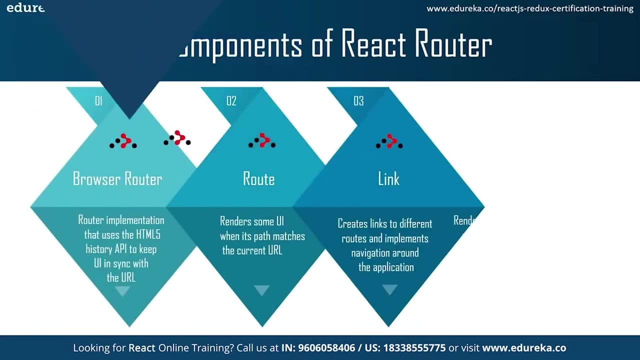 and we can just modify it and we'll be good to go. Now let's discuss the components of a react router. So there are four major components of react router which are frequently or always used whenever we are working with the react router. The first one is browser router. 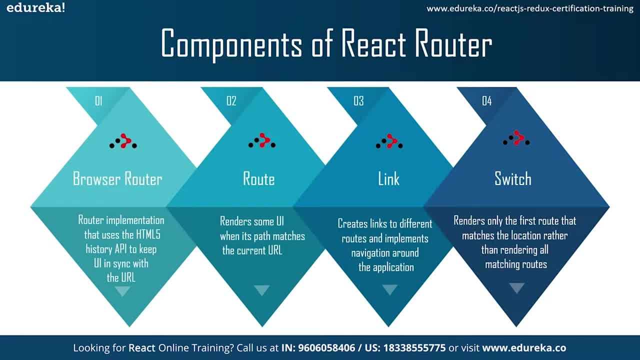 Then we have root, then we have link and then we have switch. talking about browser router, browser router is a router implementation that uses the HTML 5 history API, which includes push state replace state and the pop state event to keep our UI in sync with the URL. 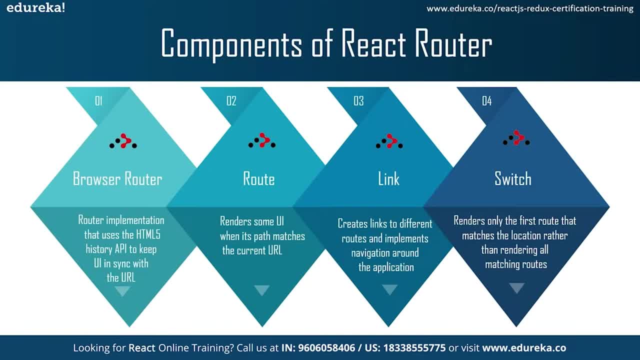 and it is the parent component that is used to store all of the other components. moving to root, So root is the conditionally shown component that renders some user interface when its path matches the current URL. talking about the link, So link component is used to create links to different routes. 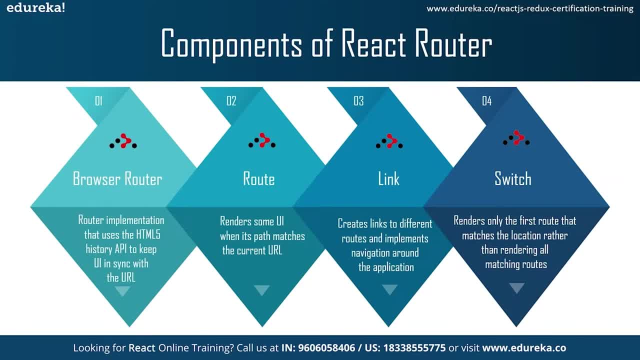 and implement navigation around the application and it works like HTML's anchor tag. and talking about the switch, so switch component is used to render only the first route that matches the location, rather than rendering all matching roots, Although there is no defying functionality of switch tag. 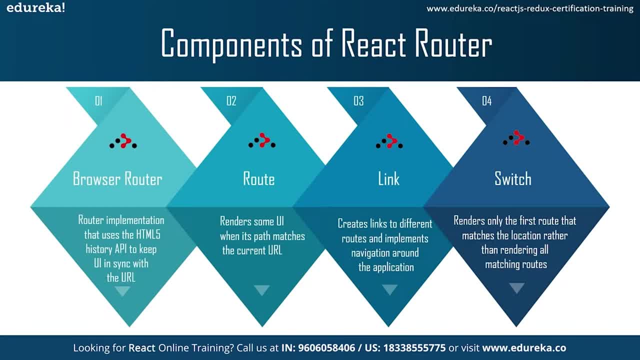 in our application, because none of the link parts are ever going to coincide. But let's say we have a route that there is no exact in here and then all the root tags are going to be processed with, which is start with slashes. This is where we need switches statement to process only one. 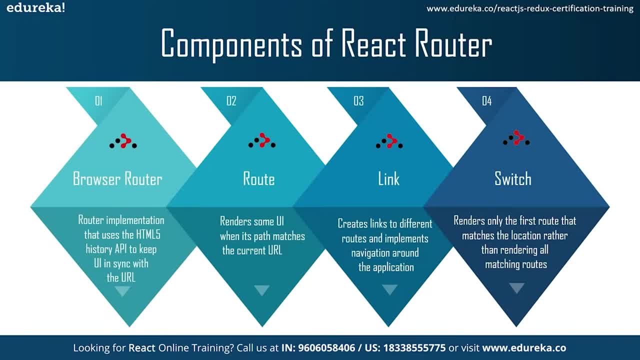 of the statements. So this we will see by a demo. So now I'll just open my vs code, the editor which I am using. you can use whichever editor you want to use, and then we'll see how to include these components of react router on the basis of the part of URL. 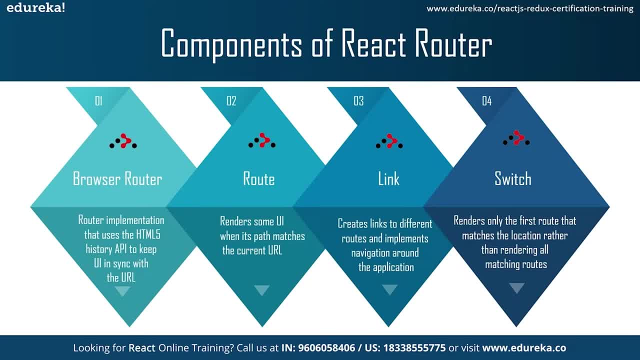 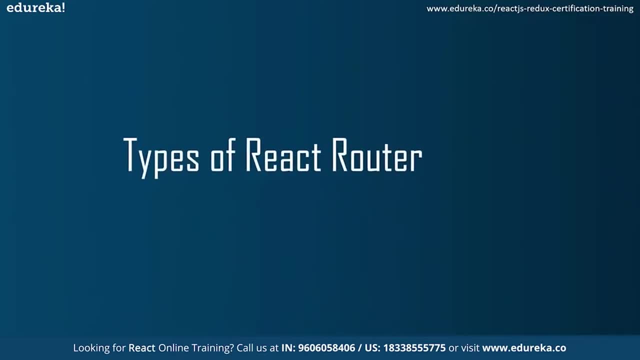 that the router will use to track the content that the user is trying to view. react router provides three different kinds of routers. Now we will see the types of react routers, So they are namely memory router, browser router and hash router. talking about the memory router, memory router key. 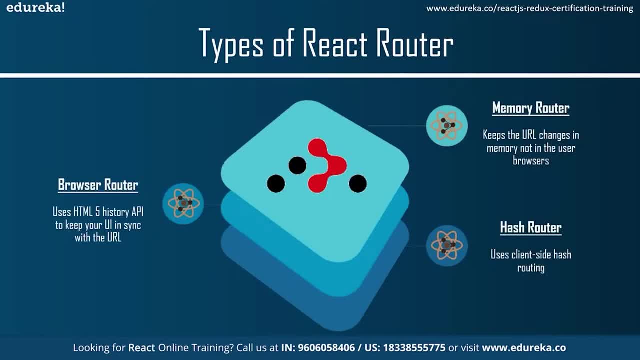 Keep the URL changes in memory, not in the user browsers. keeps the history of the URL in memory and does not read or write to the address bar. So the user cannot use the browser's back button as well as the forward button. It doesn't change the URL in our browser. 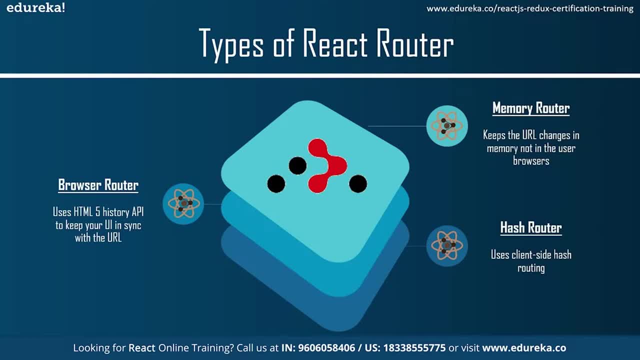 It is very useful for testing and non browser environments like react native. talking about browser router, It uses HTML 5 history API, which includes push a state, replace a state and pop state APIs to keep our UI in sync with the URL and roots as normal URL in the browser. 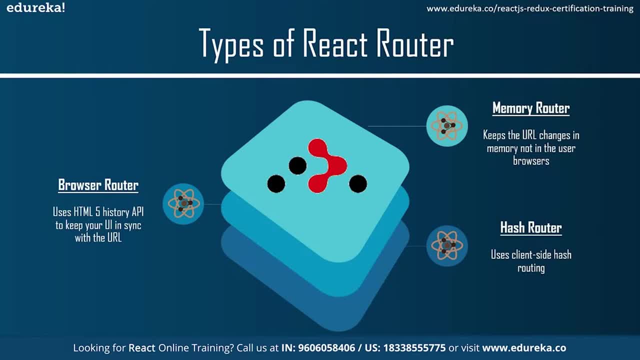 and assumes that the server is handling all the request URL and points to root index dot HTML. It accepts force refresh props to support legacy browsers which doesn't support HTML 5. pushes state APIs and talking about this, hash router. So hash router uses client-side hash routing. 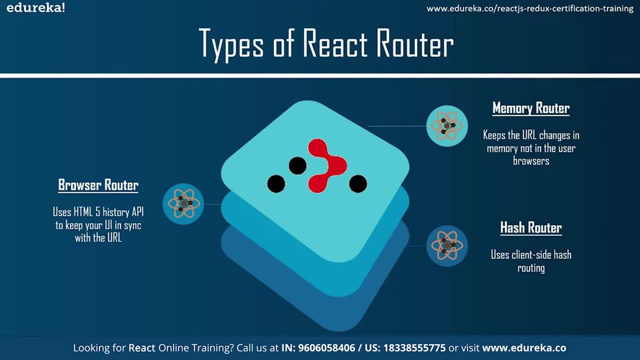 It uses the hash portion of the URL, that is, window dot, location dot hash, to keep our UI in sync with the URL, And hash portion of the URL won't be handled by the server. The server will always send the index dot HTML for every request and ignore the hash value. 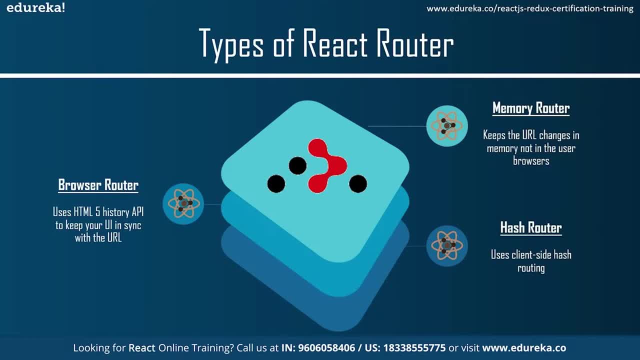 It doesn't need any configuration in the server to handle roots and it is used to support legacy browsers which usually don't support HTML pushes state API and it is very useful for the legacy browsers or we don't have a server logic to handle the client-side. 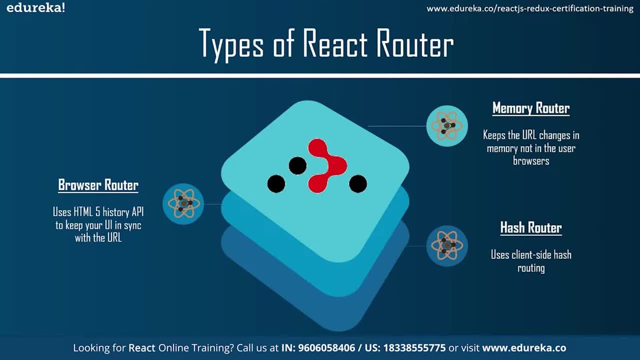 and this route isn't recommended to be used by the react router daunting. and the syntax for these kinds of router We'll see just in the import statements. We just have to change it and we will alias it as router. Let me just show you now. 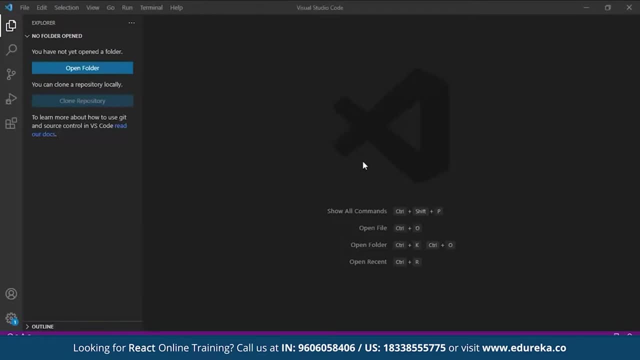 What we'll do is we will set up our react application, So we'll create a react application using create react app, and for that Let me just go to my command prompt there, Let me just go to the desktop So I'll change the directory over here. 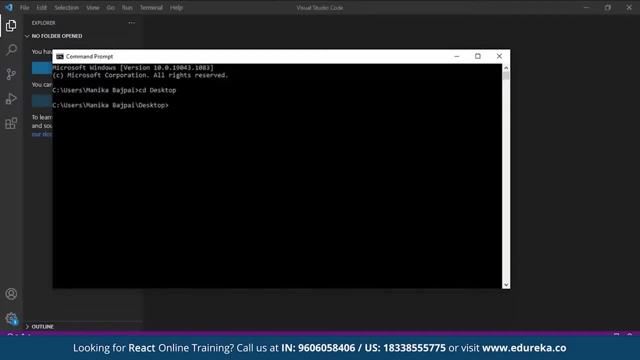 I'll move to desktop and then I'll run this command: NPX, create hyphen react hyphen app, and let me call this app as edureka routing Now this command will create. So now here you can see, is we cannot create a project name. 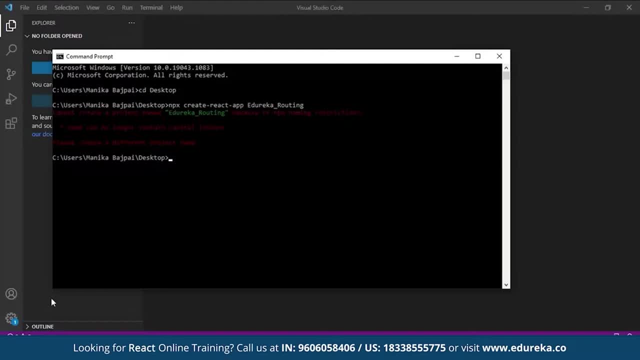 edureka underscore routing. because of the NPM naming restrictions, name can no longer contain capital letters, So I'll just give it as edureka routing. Now, here you can see. we're creating a new react app in this folder. Okay, inside the desktop. 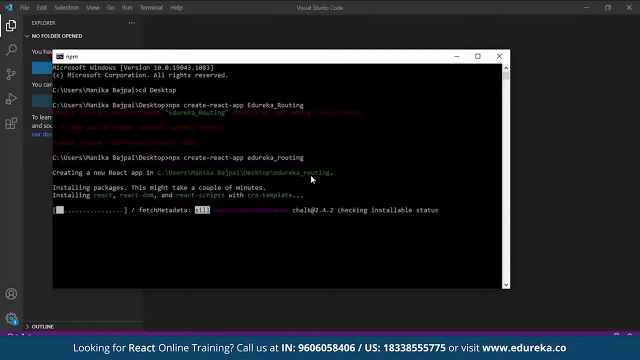 We'll be getting folder for react application that will be known as edureka routing, and it will take some time. It will actually take some time, like around two, three minutes, and once this will be done, then what we'll do? we'll move to our this application folder, that is edureka routing. 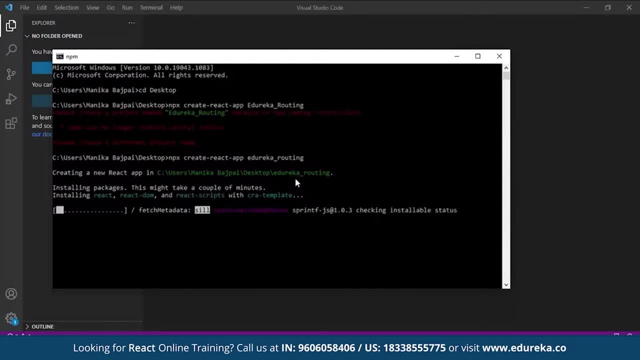 and then we will install our react router Dom, which I had explained you. it contains the Dom bindings for react application will make use of NPM And we'll install react router Dom and then we'll start adding the components. I'm using the visual code, visual studio code, as editor. 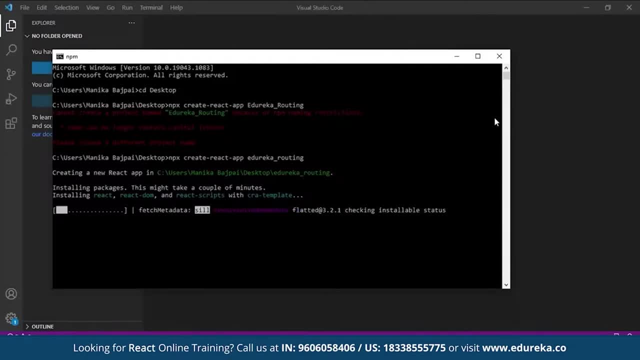 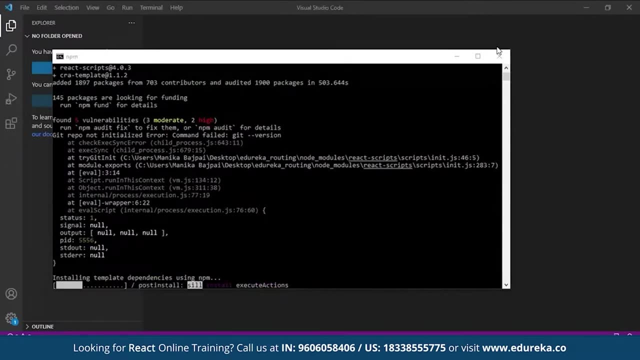 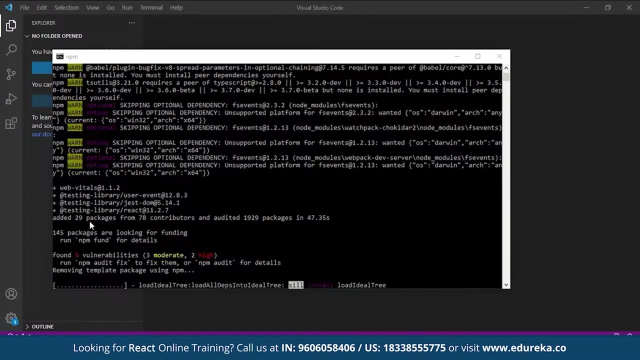 You can make use of any other editors as well. Now, as you can see, the dependencies have been installed and you can see over here as well, like some 29 packages have been added. so with this create react app, we can simply create our react application. 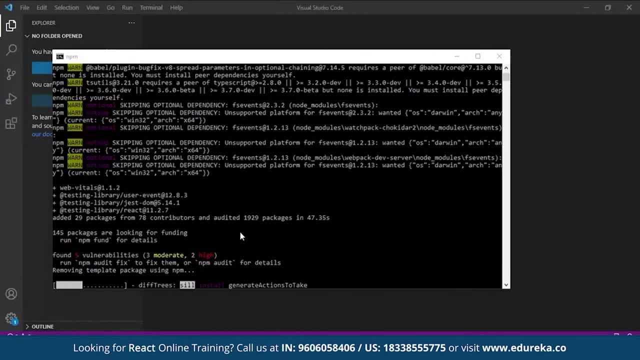 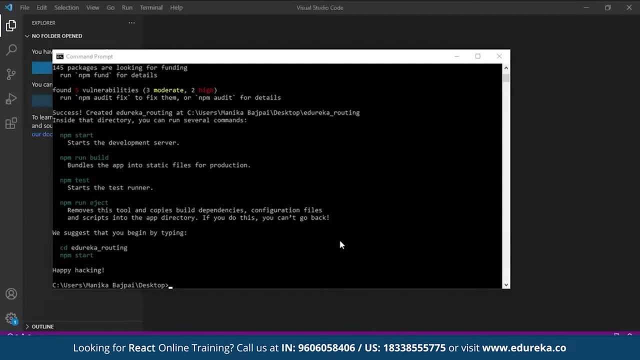 and we can just add the codes, we can add the components and we'll have a react application created. With this, we have successfully created our react application and the name of our react application. We have given us a direct routing. Okay, as we are going to learn routing with this, 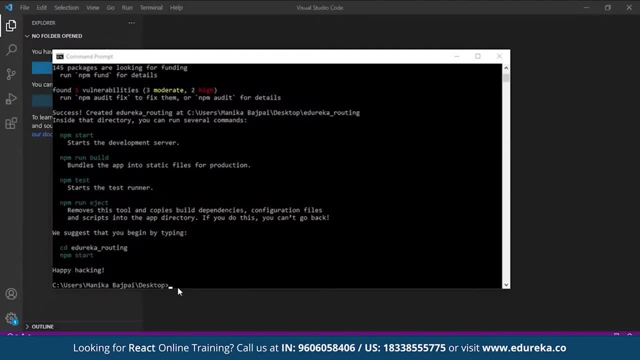 So with this you can see over here happy hacking and now we are good to go. Now what I will do is first we will move to the project directory or the application directory which we have created. right now We'll give CD and edureka underscore routing. 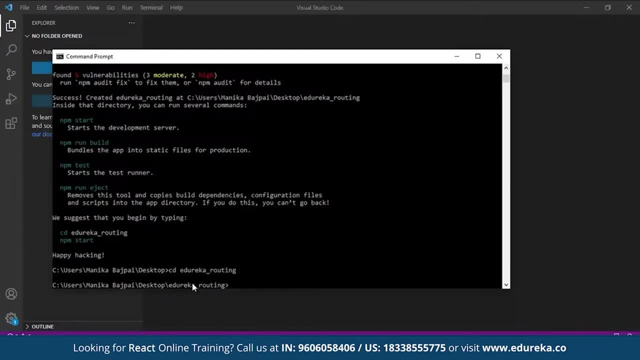 and now what we'll do is we will install the react router Dom for our this application. So we'll give NPM: install react router Dom- Okay, router Dom. and we will give a space and hyphen. see this command. We have to give all right. 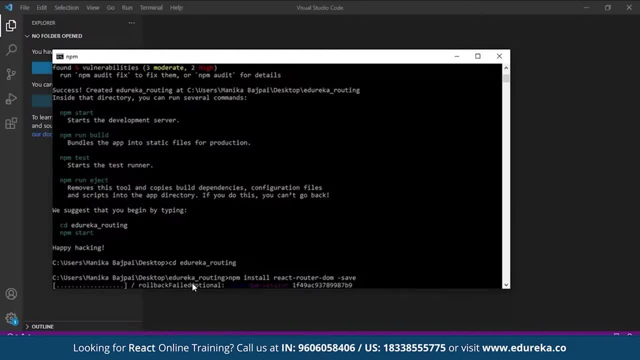 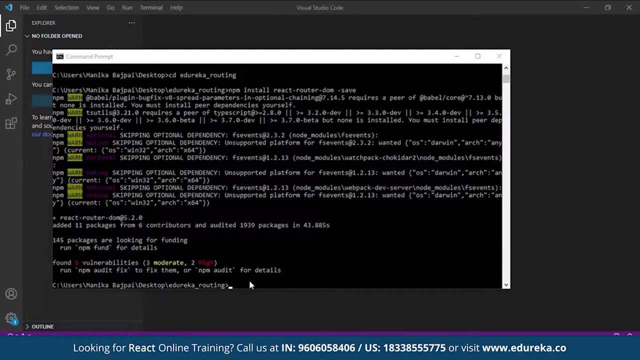 This will install our react router Dom for our existing application, which we have just now created with the help of create react app. It will also take some time, but less than the previous one. And, yes, with this we have successfully installed our react router Dom for our edureka routing application. 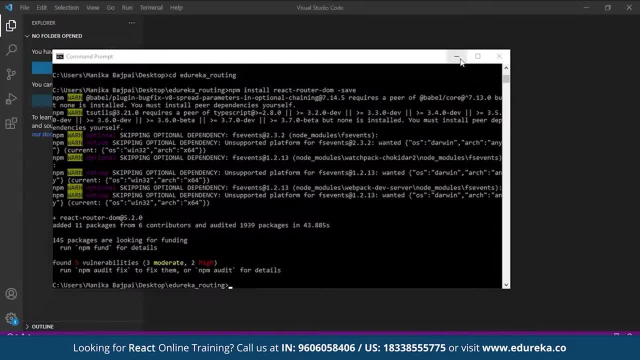 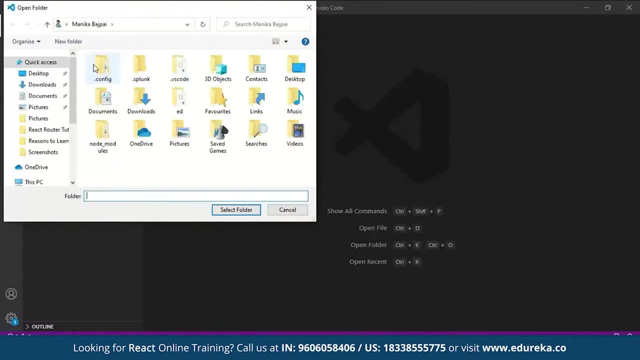 Now what we'll do is now we will start creating or adding the components to the application. Now what we'll do is I'll just close this up and in my vs code I'll open the folder which has my application. So in this, yeah, in desktop- 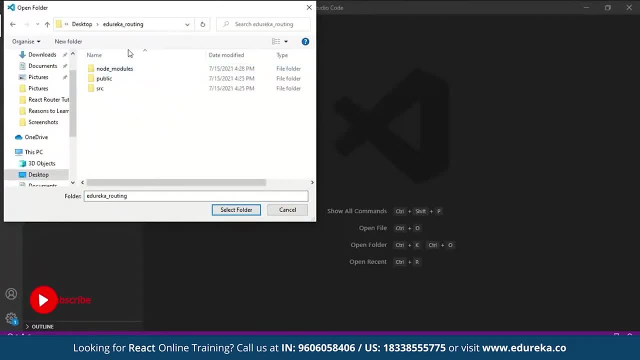 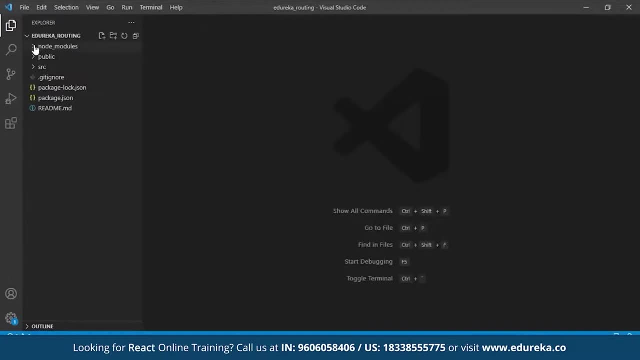 you can see, edureka routing is there and they just open this one. Now, here you can see our application, or the main folder is edureka underscore routing. Then here we have node modules. all these libraries and the dependencies are here, like you can see, Babel. 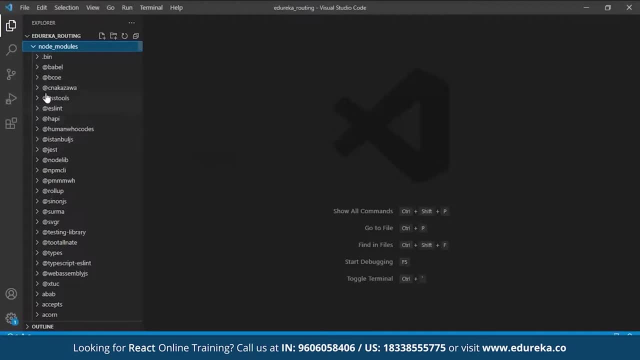 and all for es6 and all we have just for testing. So all these are available. They have been automatically added with the help of create react app and then here in this public we can see. here is the index dot HTML. So if you want to change the title, 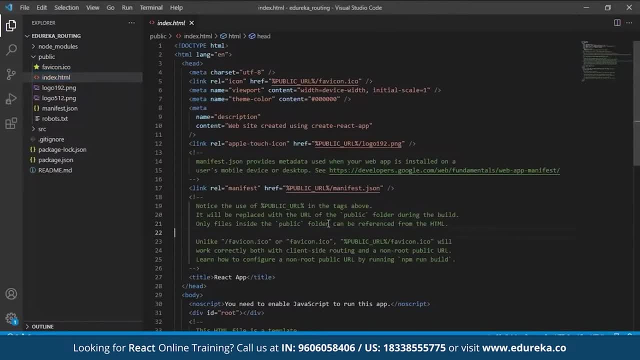 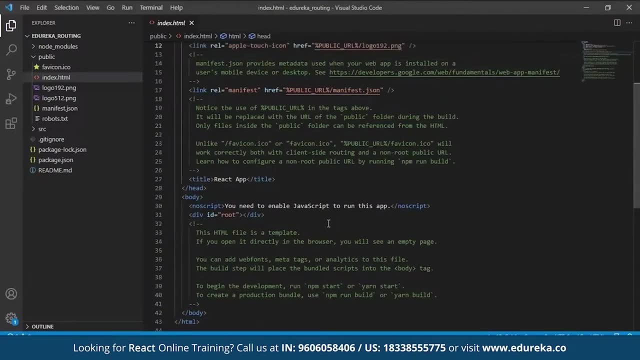 or the HTML part of our application. we can just make changes over here, or we can just create the new one. We can just create a whole new code as well. So I'm not going to all these HTML and CSS part, naturally, because we are here to learn about routing first. 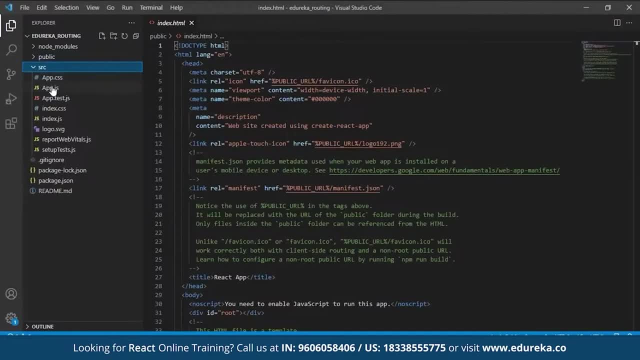 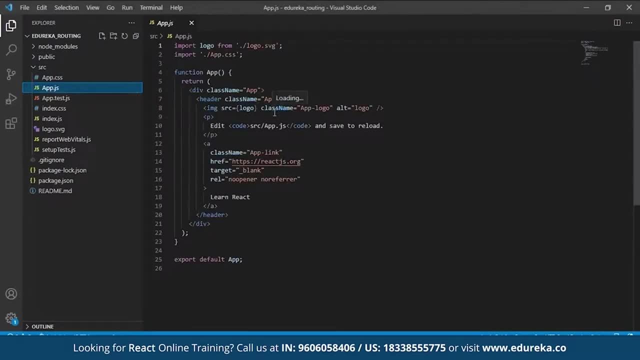 What we'll do is we'll go to our SRC folder and here you can see we have appjs file. So this component, this is actually where we will be using router react routers. We are going to make use of them over here in this application. so that will provide the links. 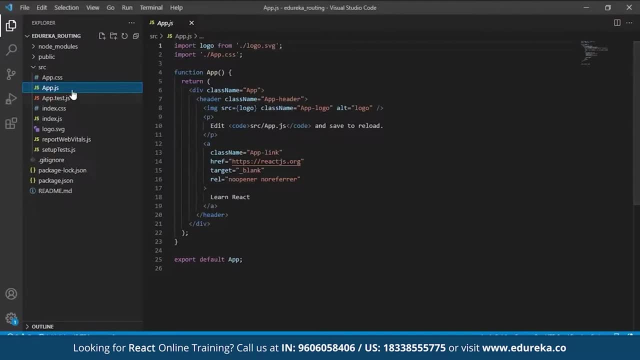 and the switch and everything Which will be linking to the other components. So what we'll do is, first of all, let me just remove a whole code because this is a default one. This create react app is for the default one. It is like reacts- default application. 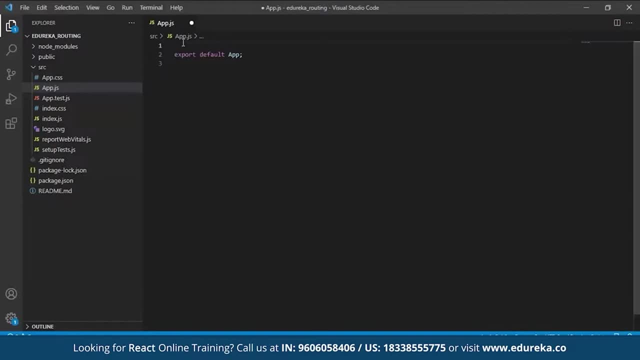 which has been created. now We have to create the components at them with the help of routers and all. the first, what we'll do is we'll import our router. So what we'll do is we'll write import. So, as we have learned about the routers, 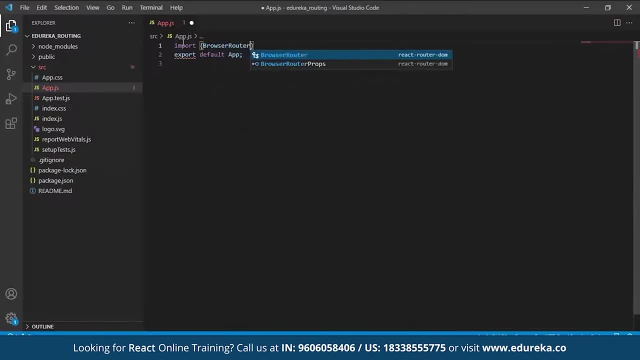 so we'll give browser router. as we have seen, This is the first component of react router. So we'll give browser router and will alias as router. Then we have the other component, that is, root, Then we have link and then we have switch. 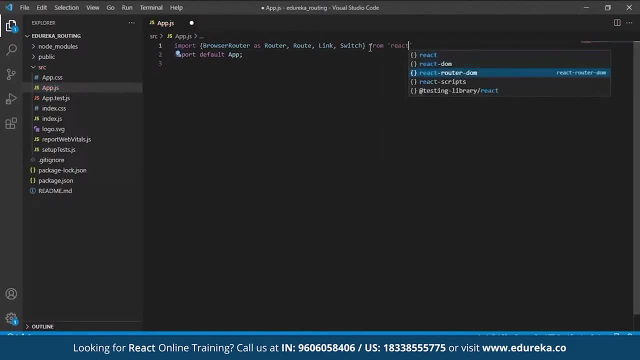 and this we have to get from react router Dom. Now here be clear with the thing that here this browser router is aliased as router. now to use react router, What we'll do is we'll create components in this react application. So what we'll do is, inside our this SRC folder. 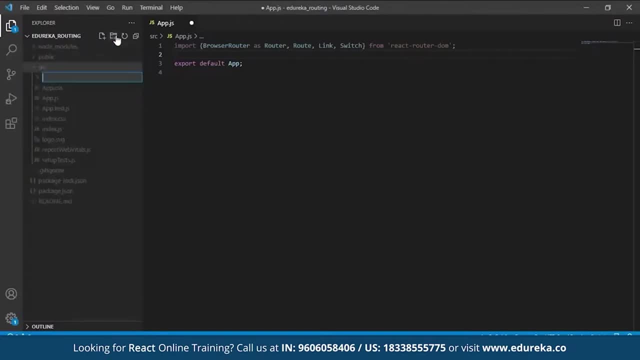 What we'll do is we will create one more folder and that we will make it as component. So we have one more folder inside the SRC that is component. Now, here in this will create other files, other JS files, which are actually the components. 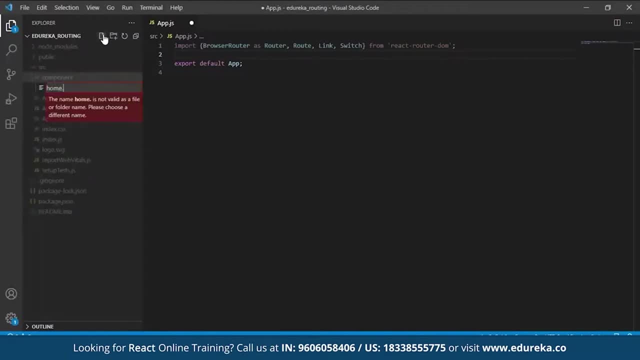 So let me just add one file as homejs, then we will create one more about dot JS, and then we have contactjs. So these three components I have added. now let's add some code to this so that will be available on the screen whenever we will be executing our application. 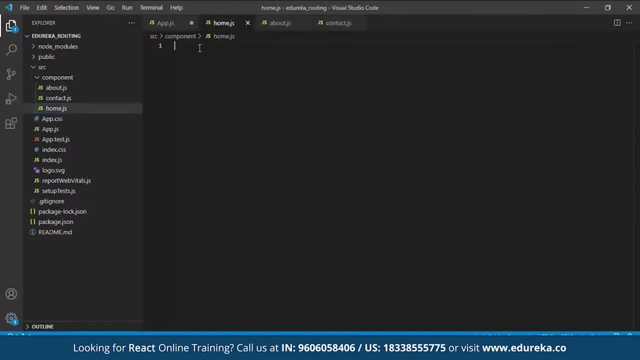 So let me just go to home and let's add some code, Like: first thing is we have to import react from react and then we will write the function or the reducer- We know function home- which return heading will write like: welcome to at Eureka. 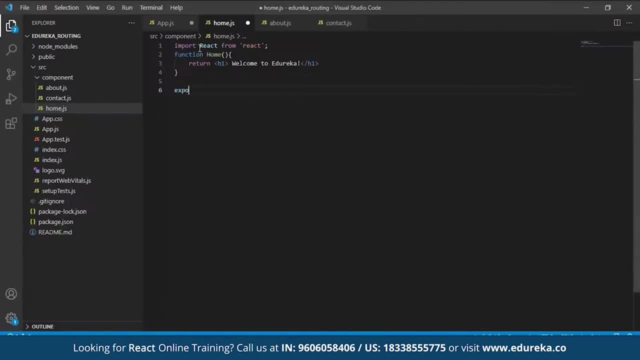 and that's it. and then we'll close this function and we'll write this export default, app default. We'll just save it and then next is our about component. So in this will simply let me just copy it from here, We'll just paste it and we'll make the changes over here. 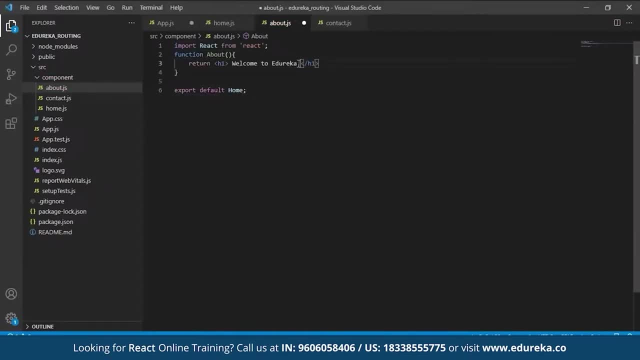 Here is about now, Let me write. Let me write something about at Eureka. So at Eureka is an e-learning platform And let me give you some more thing. like like no more about at Eureka here. Now, here will I'll make use of the anchor tag. 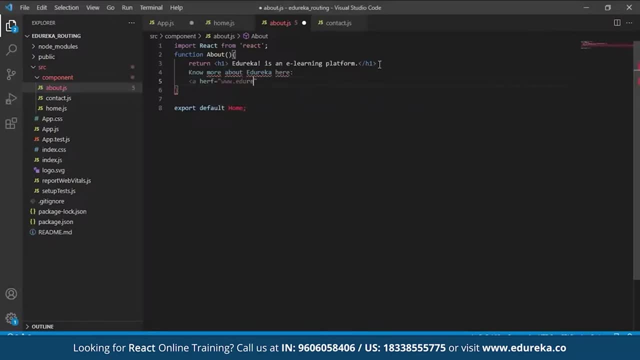 and I'll give the link: wwwedurekacom. Now, here we have the link, and I want to display this as well. So what I'll do is I'll just type it over here as well, And with this we have closed our anchor tag. 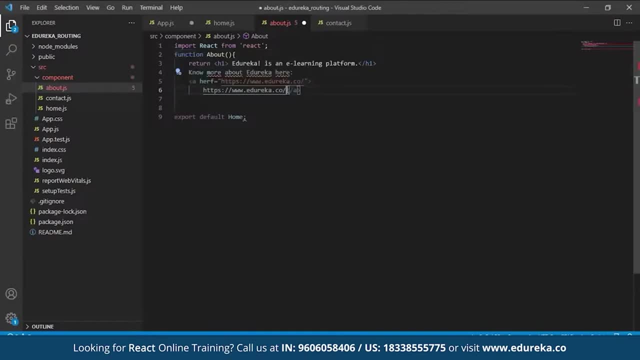 Now, when we have created this one and the anchor tag is closed over here. Now one more thing is we have to return something. So here in return, I'll put all this inside our div. So this one is also ready, and here I have to give this about the function. 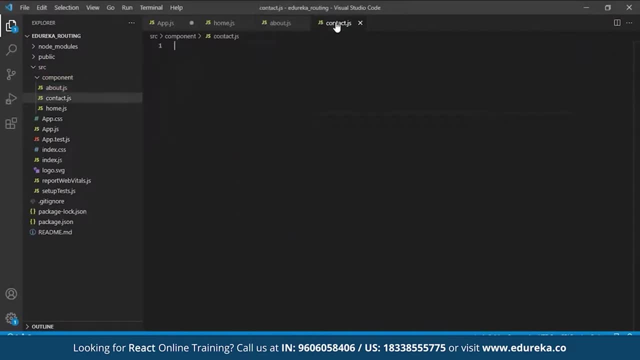 which we have just now created. Let's save it. and now, moving to our contact component, So again, let me just copy this thing and we'll put it here now. here, What I'll write is like: for queries, contact people: No, no link. 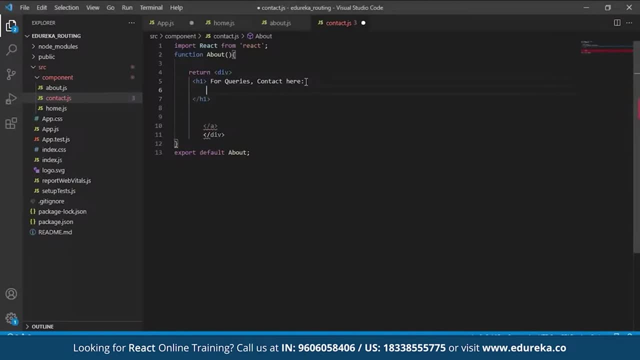 I don't want to give any link over here Now. let me just the number, Let me just put this over here. and one more thing, see, and if I want to put it in the next line and all so I can just give the BR tag, as we know in HTML. 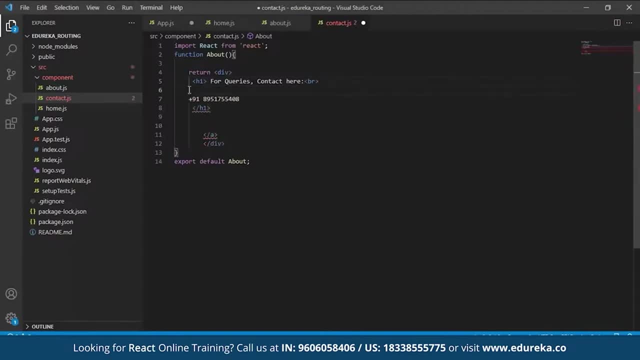 and no need to give it like this. Let me give one more Yep Now in this. about what we'll give is we'll get the in place of about will give contact, which is: remove this anchor tag. Now let's make a little change over here. 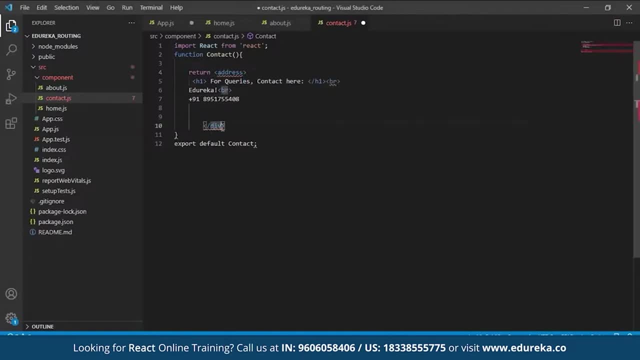 Let me just put it inside the address so that it will be like a single element over here, and let's just remove this heading tag. All right, and we'll just give it up. So we have created, created three components and we have added them. the home component: 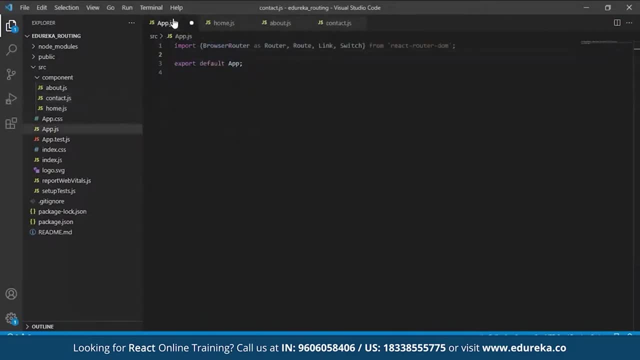 and about component. then we have our contact component now in this appjs. What we'll do is we will make use of our react router and then we will link these components. Now what we will do is we will start adding the components to our appjs- the components of react router over here. 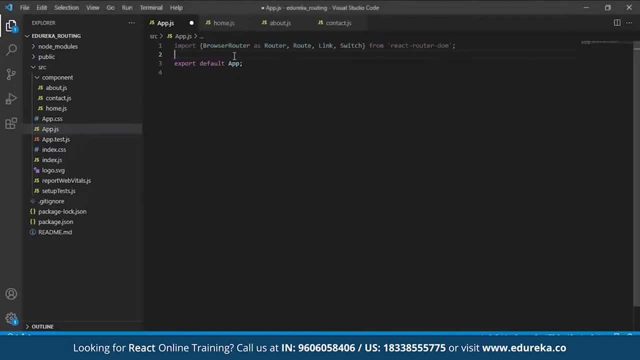 Now, as we have already added this browser router as router, Now let me just create class app Extends component and then we'll give it as render. make use of render function that will return router and inside a div, provide the class name. give it as app. 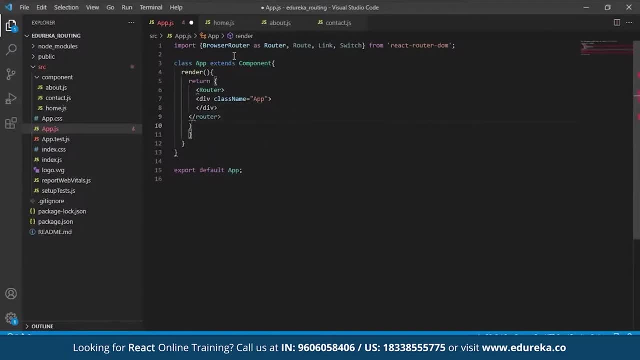 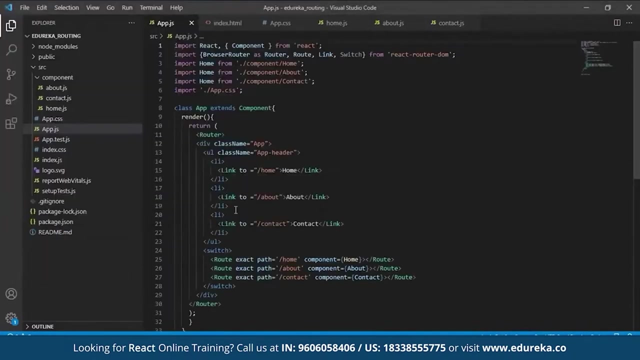 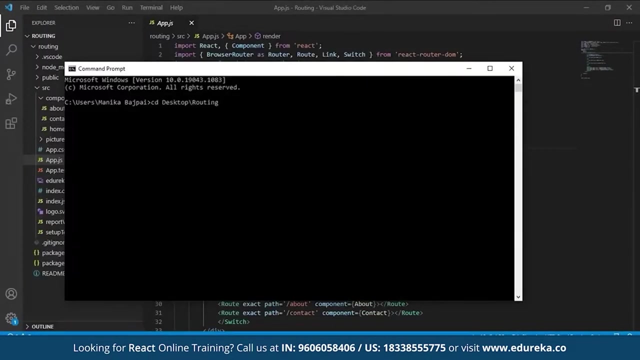 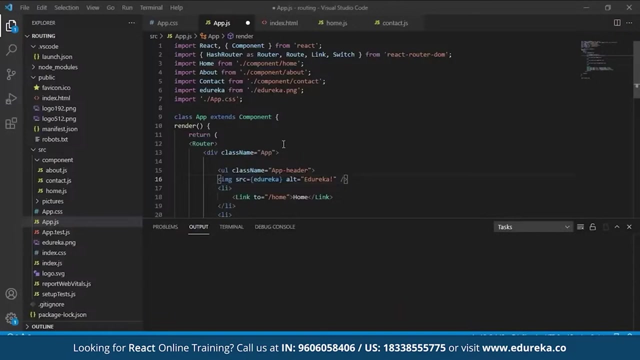 and then we have closing tag for a router. Now moving ahead, What we have to do is, inside the div, we have to put the links as well. link is also one of the component of react router. before moving ahead, We can just see. let me explain you the components. 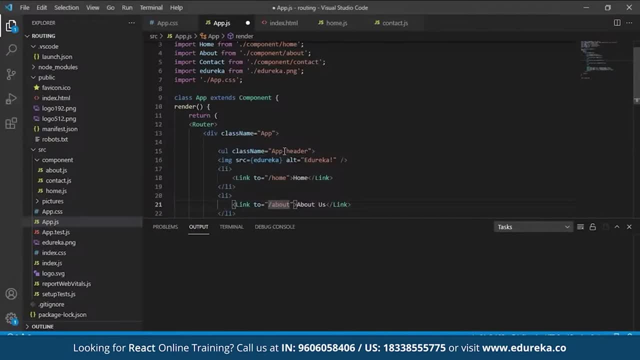 which we have created, especially talking about the props associated with the root component. We'll see over here, as you can see, the exact right this: this is used to match the exact value with the URL. For example, here we have given exact and then the path. 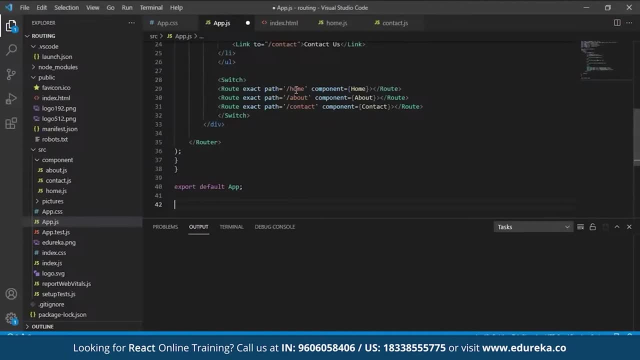 that to home component and this will only render the component if it exactly matches the path. if we remove exact from syntax, then UI will still be rendered, even if the structure is like slash and home, like that, and then we have something called is path over here. 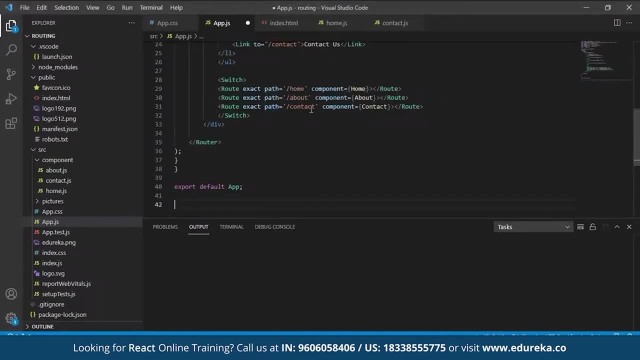 So this specifies a path name we assigned to our component, The path name which we have assigned, like contact home about like that, and then we have something called as component. It refers to the component which will render on matching the path, these components which we already have. contact home about all these. 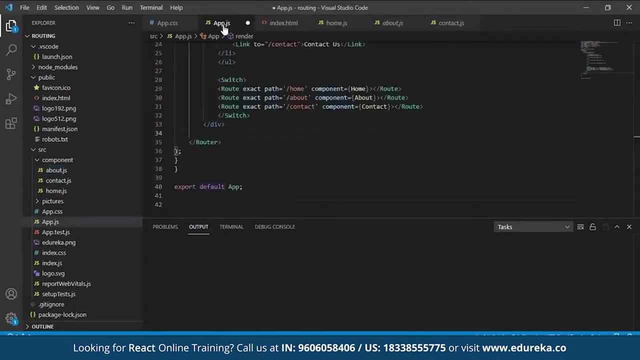 and, as we have seen in this, we have switch as well. This switch will be used to render a single component wrap all the roots inside the switch component. So we have just wrapped it around and this link we have used to create the links to our component. 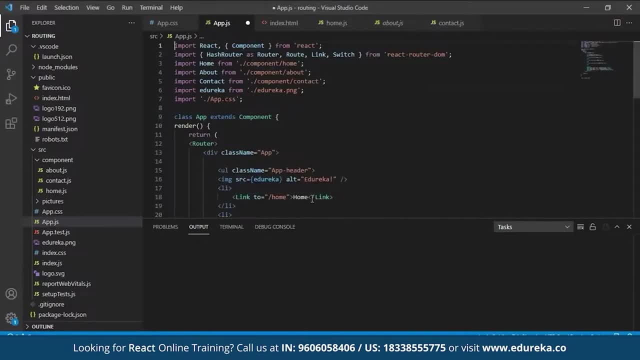 It uses the to prop to describe the location where the link should navigate to. so here you can see this to prop. this to prop has been used by this link component. Now let's see the output of this application, or this code which we have written now. 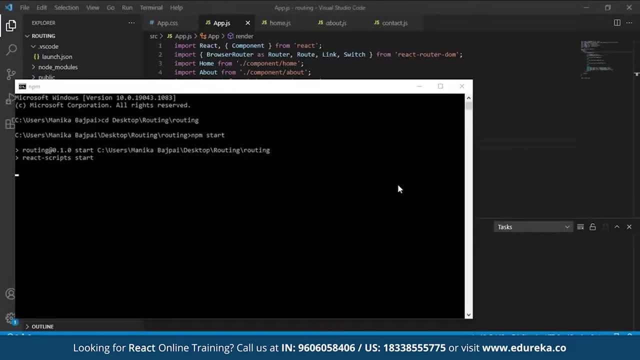 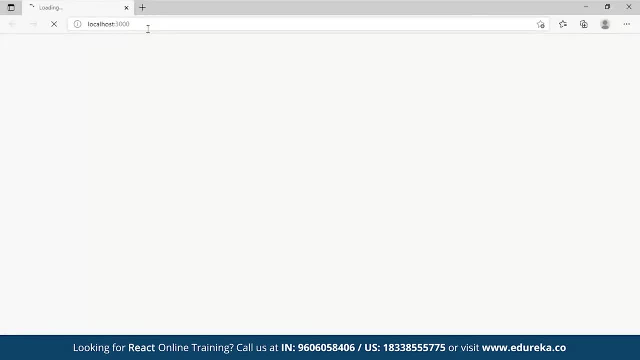 We will see the UI of our application, taking a little time So it will get executed. browser will be launched here So you can see over here on localhost 3000. It will be launched here. It comes now. This is the page. 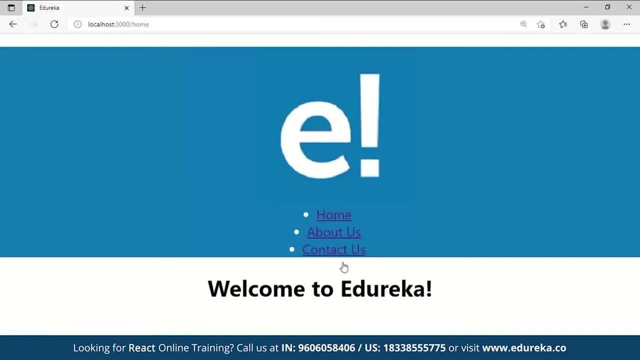 Okay, Now, whenever I'll click on home. now we have moved to our home page. This is happening with the help of a router, the components which we have used: the link component We had made use of, browser router and the switch. now, when I click on, about us here. 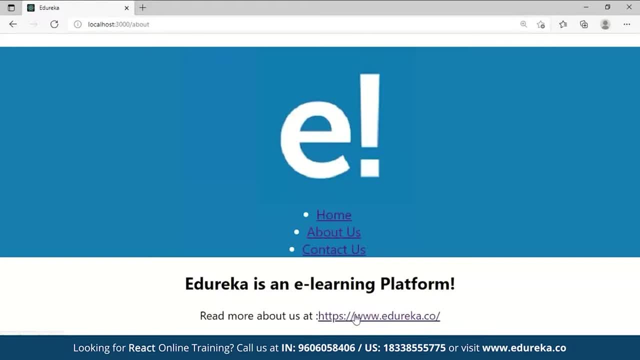 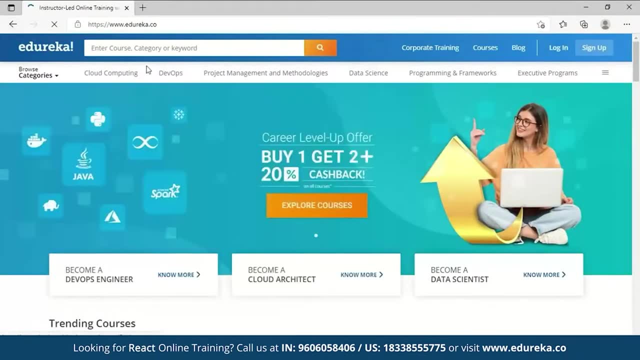 you can see the URL is also changing and with this if I click on this link. So this is the normal HTML link part. with the help of anchor tag. I have just redirected to our edureka homepage. Let's go back and then on contact us. you can find it over here. 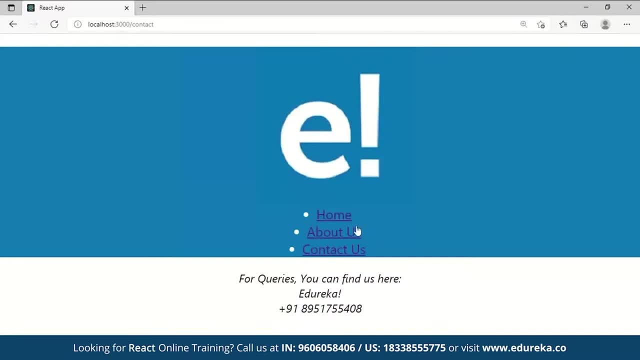 So whatever we wanted to display in our application, that's being displayed in the different pages and we are redirecting to these pages with the help of react router. and here is the URL, and the application name is like react app. We can make change in that also.